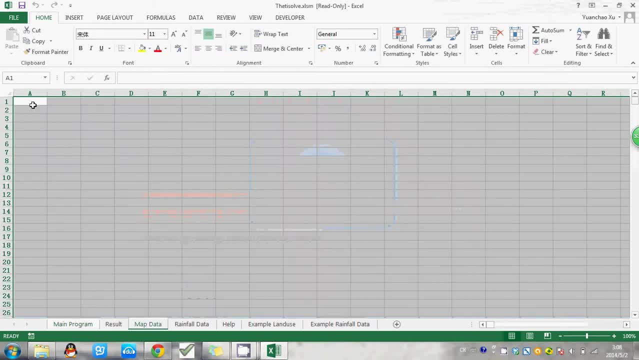 the worksheet Map data. Click OK will be there. Okay, And because our model is a bugging model and the model's principal is that you have to have a rainfall and you have to have, you have to have your land use map and use the rainfall and your land use map. 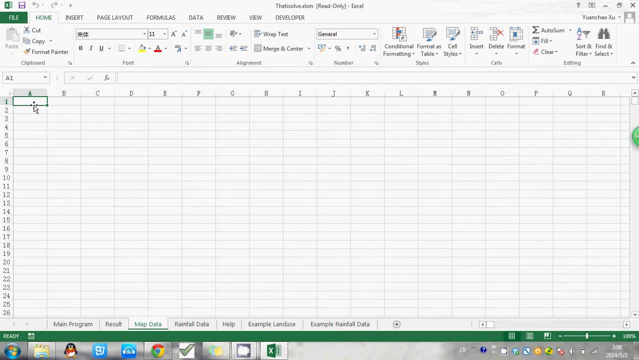 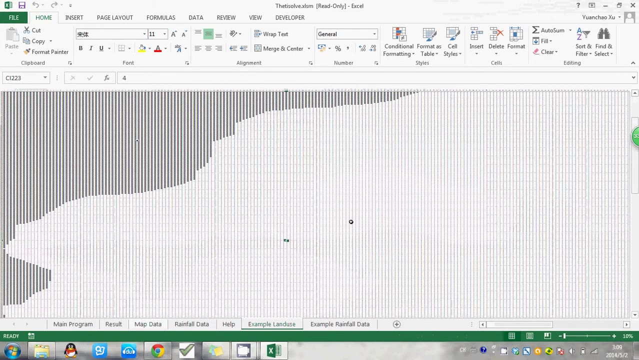 to generate the runoff of the catchment. so first of all you have to have the information about your catchment. that means you have to have the map data. in this case it is the land use data. don't worry, we have examples for that. we have examples of the land use. but you know this catchment is big and have like a 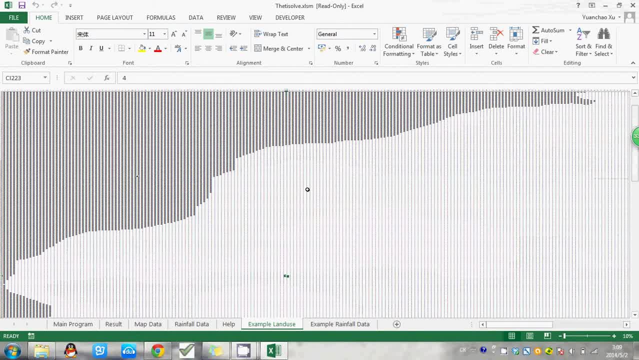 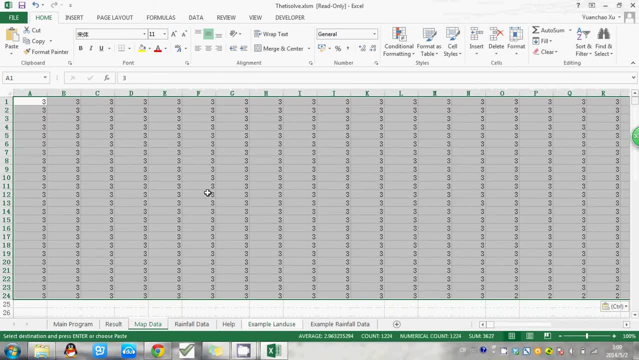 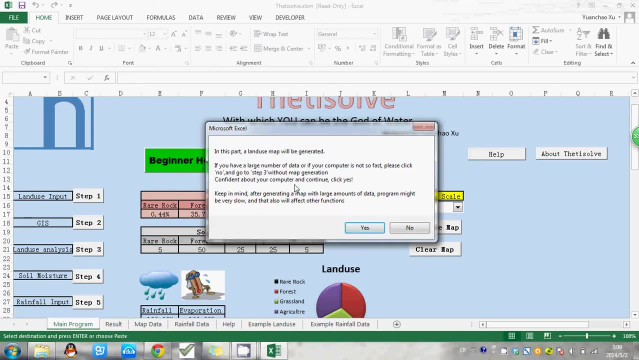 lot of dangers because, for example- which is true- that's more part of it. copy paste here. okay, and then go to main program, step 2. you will see that if you are have a large number of data or if your computer is not so fast, just click no. 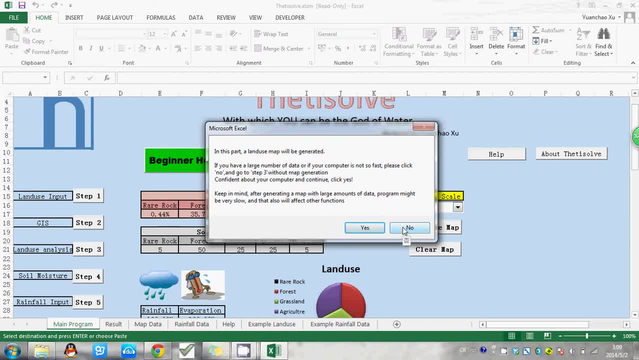 and go to step 3 because step 2? the difference between step 2 and step 3 is that step 3 won't generate map using Excel and your computer will be like much faster if you don't click step 2 but in this, then in this example we only have a smaller kind of part of data, so it's 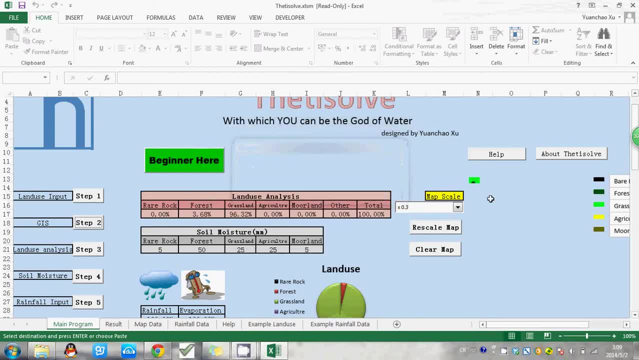 okay to click yes. then you will find: okay, the map has generated but it's just too small. you want to see the details you can here. we have map scale. you change it to two and rescale map. see it is bigger and you can see that the map is. 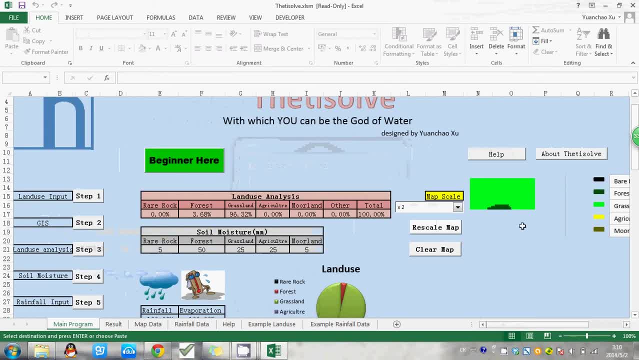 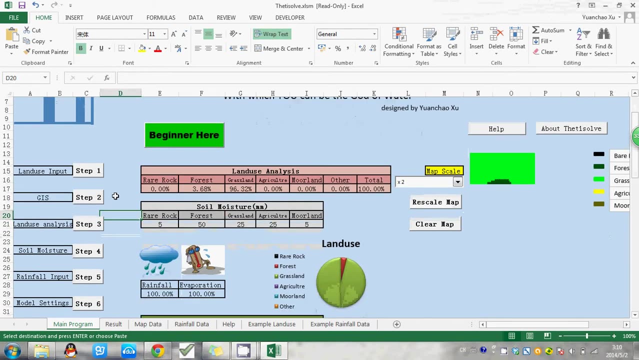 bigger and you can see the length in here. this part means forest and this part means grassland. also step 2, step 3 actually just executed the same function and because we have already used the step 2, we don't have to use step 3 and at 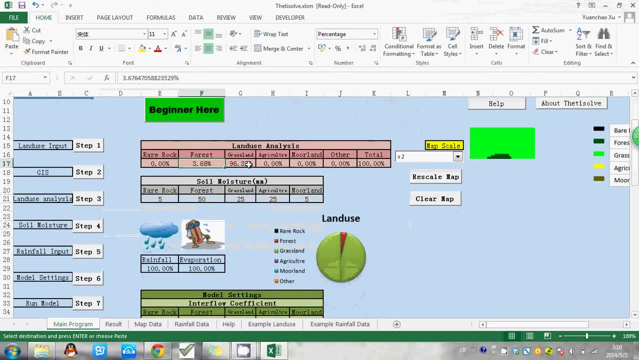 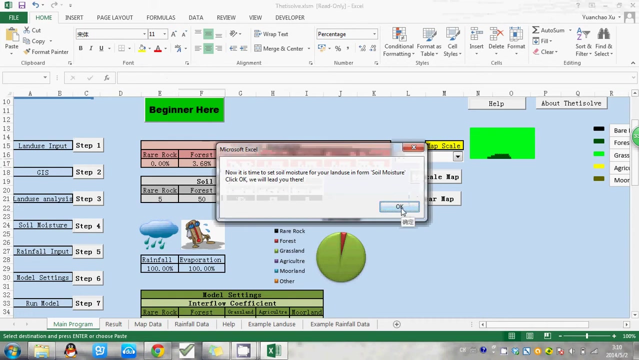 the same time, you can notice here the number changes because we have already analyzed the data, the land use data that see, we have like three percent of forest and 96 percent of grassland. I can, you can, see the distribution of land use here and then we'll go to step 4. it's time to set the soil moisture, which is also. 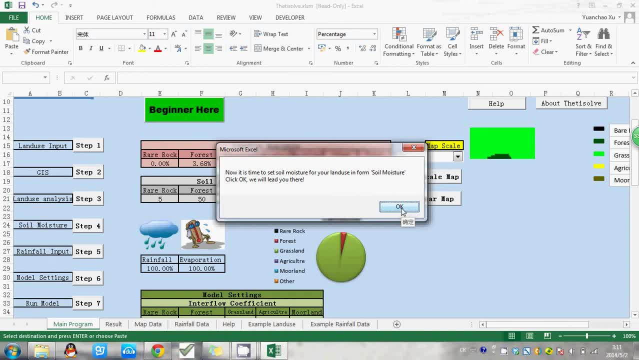 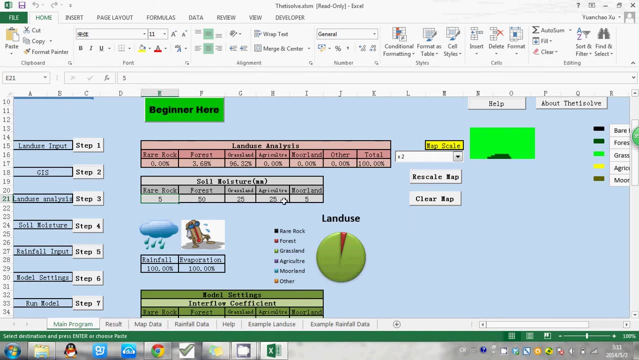 means fuel capacity in the bucket model. okay, you can see the cells here and selected. different land use has different soil moisture in this guy. you know the default number is 5, 15, 25, 25, 5. you can change this number as you like. maybe you? 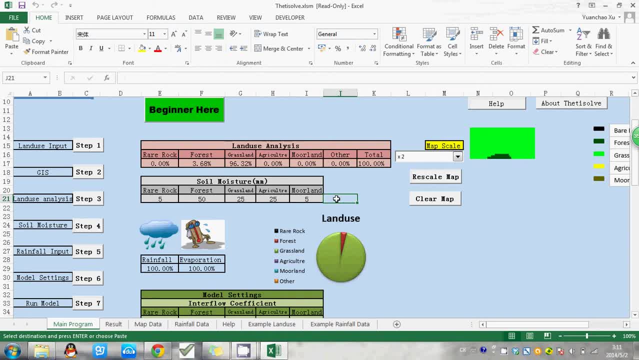 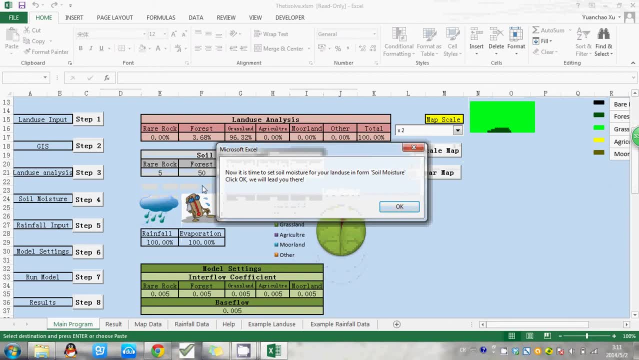 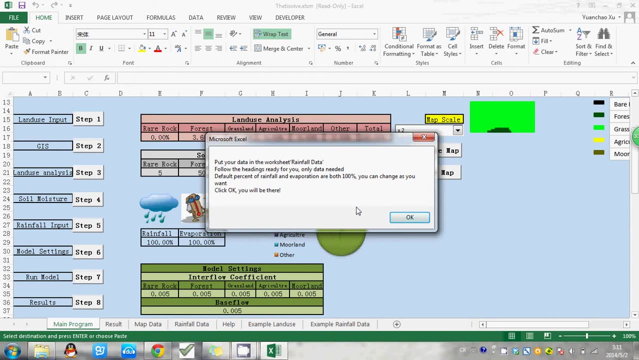 have read some articles and you think this number is not appropriate for your case. you can change it, that's okay. and also step 4. oh, no, no, sorry, step 5. okay, step 5 is the rainfall data and, as I said before, we used the rainfall data and the map data to generate runoff. now we have already got the map data and 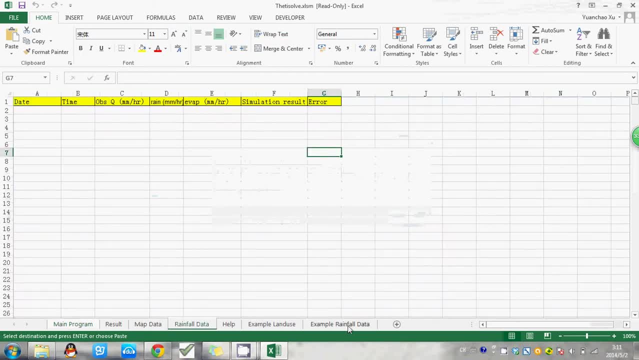 now we need the rainfall data. but don't worry, we also have examples here. first you will see, we'll put your rainfall data here. we have headings. you don't have to replace the headings because the program will start to calculate from the second row. it won't take first row into consideration. 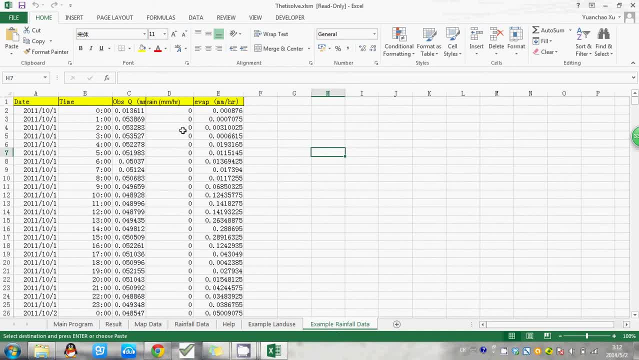 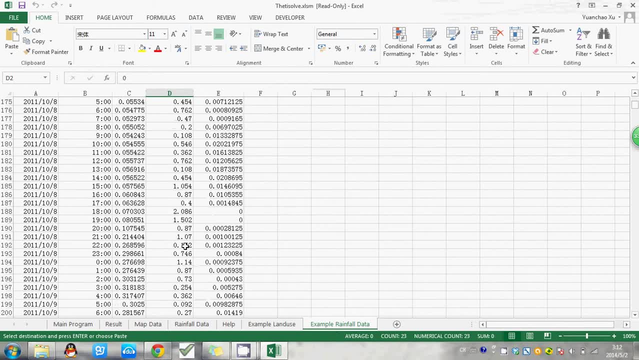 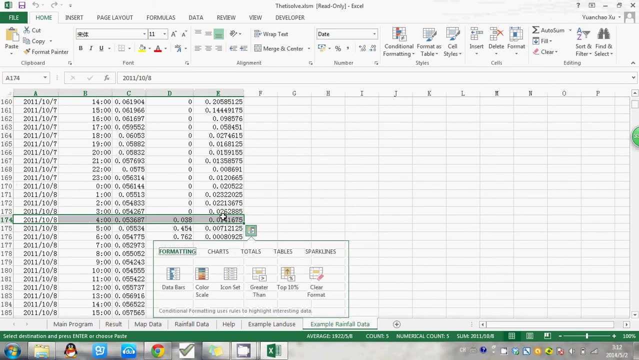 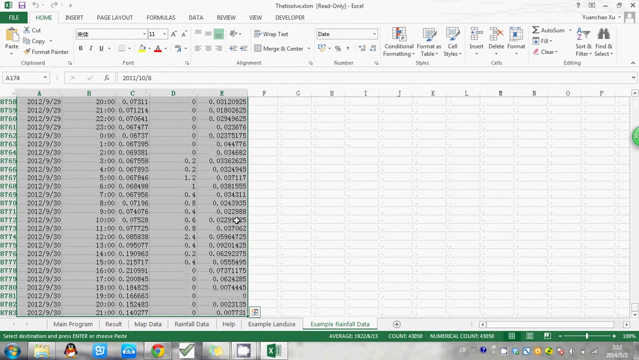 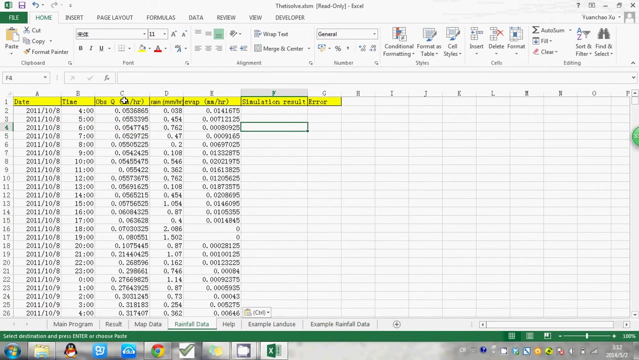 we've got example rainfall data and because you can see that the first part of the data, the rainfall, is just zero, zero, zero, which was uh, yeah. so okay, from here copy paste: okay, we've got rain, we got evaporation, we got observed data to calibrate the model. Now it's step 6. 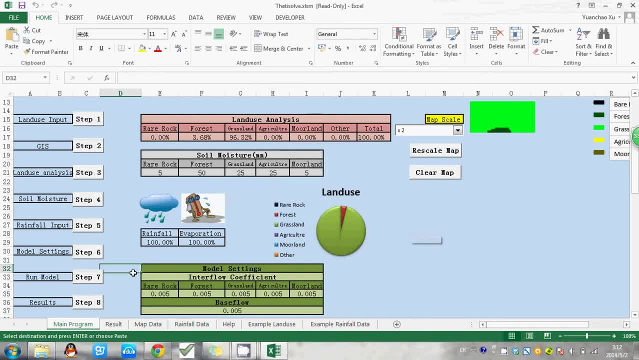 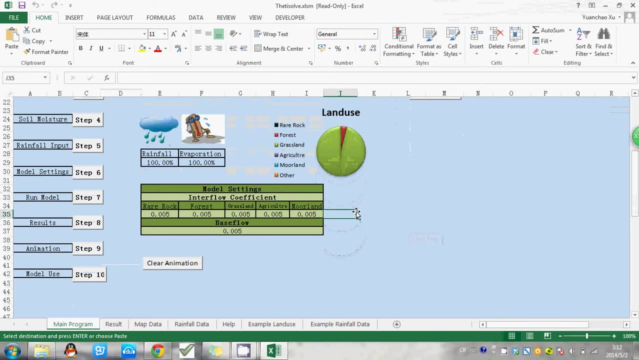 model settings. This setting is mainly about that. okay, you can see the cells here. The interflow coefficient, which means that there is some interflow between the buckets, like it's. you have to use the coefficient to multiply by the depth of the bucket and then got the interflow. So in this, 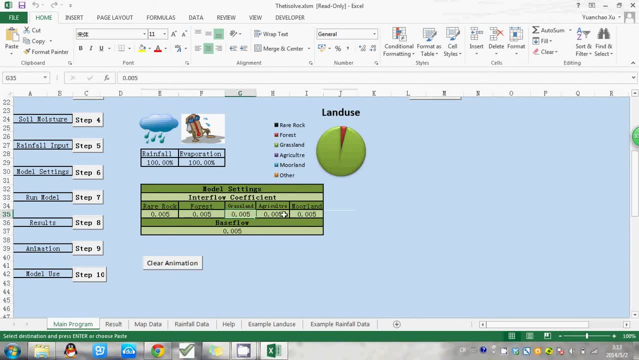 case, we have numbers for this coefficient. It's all default numbers. If you want to change as you like, you can change that For base flow. I know maybe you have different ways to calculate base flow, but in this model we use base flow for all the lunges. If you want to change the calculation method, like if: 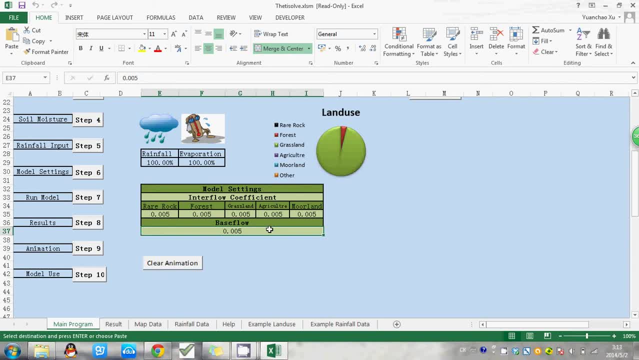 you. I have a better one and I have more suggestions about this. just email me and I will change this for you, And that's it You can like. for example, we change this to 0.04 and now all the settings has been down and we just run a model. You can see it's very fast. Now comes to 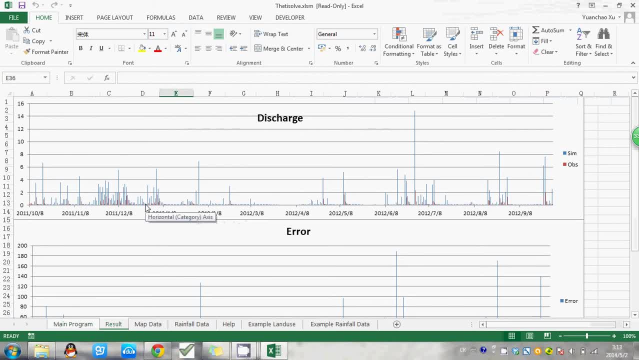 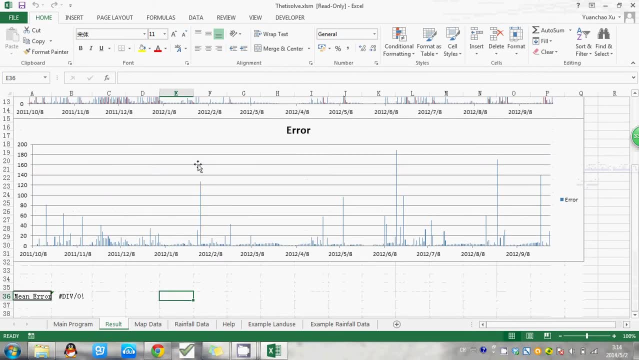 step 8 to show the result. okay, you can see the result here. the blue ones it means the simulated data and the red one means observed. the data also have errors. I just randomly choose some rainfall and randomly choose part of the land use and also just 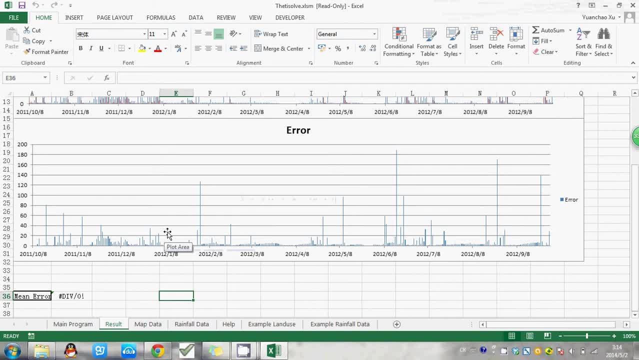 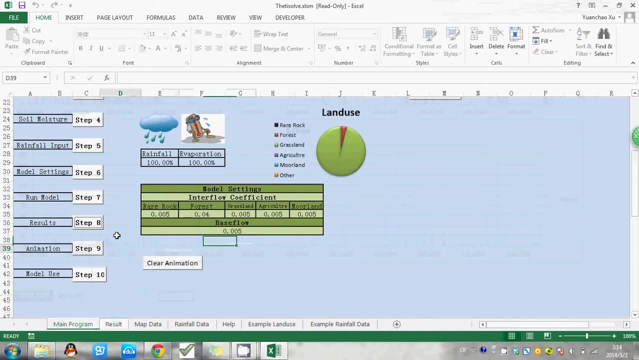 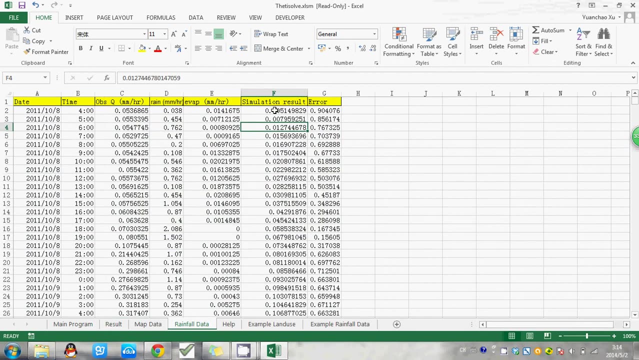 all by default numbers. the error is not so small, But after calibrating the model I think you can get a more accurate result Here. you have already. if you want to see the detailed data, you go to rainfall data, as you can see the simulation result. you will find the result here and error is here. 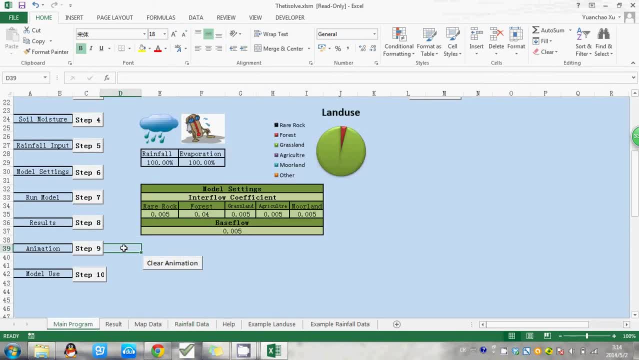 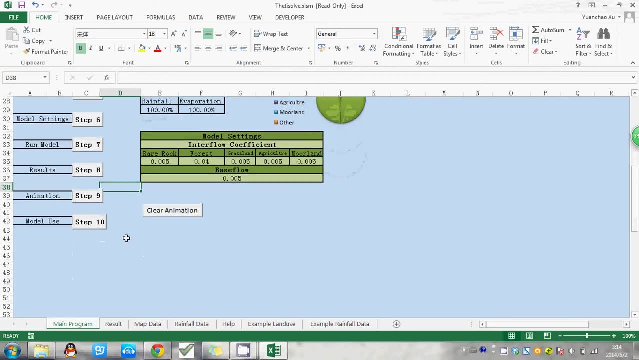 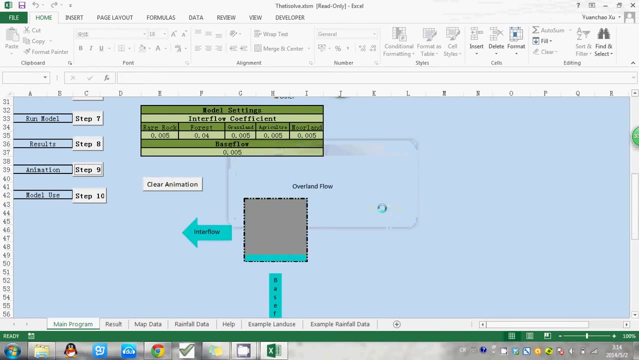 And now I have finished all part of the model, but we provide animations for you to see how it works. You can click here. ok, this is the bucket model. You can see that the interflow between the buckets and the base flow always exists. 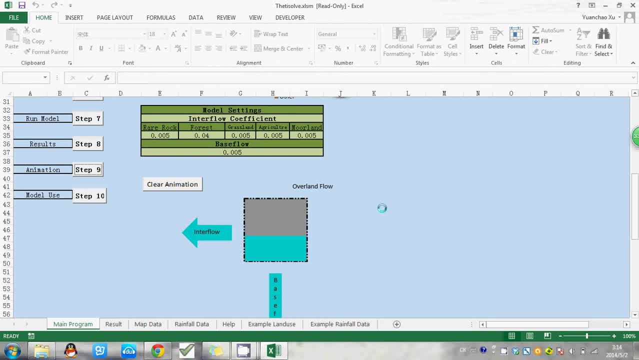 But the interflow. when you have water depth in the bucket, there will be an interflow, and when the water depth is zero in the bucket, there won't be any interflow. Also, when the water depth exceeds the height of the bucket, there will be overland flow. 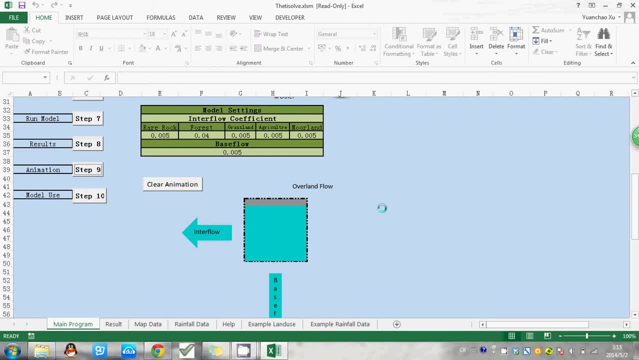 I think soon you will see the effect like there will be some water exceeds the height of the bucket. that water is changing. Ok, it's almost full. Ok, Ok, see, it exists. the height of the bucket and then overland flow generated. 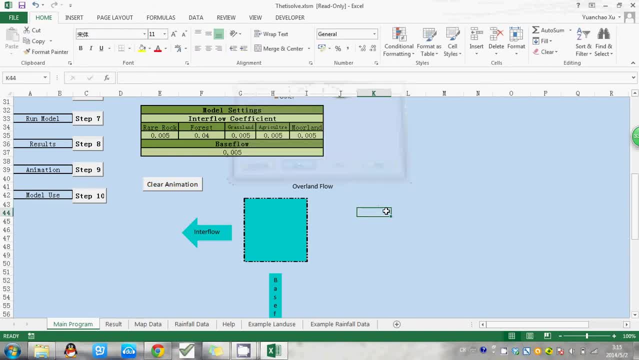 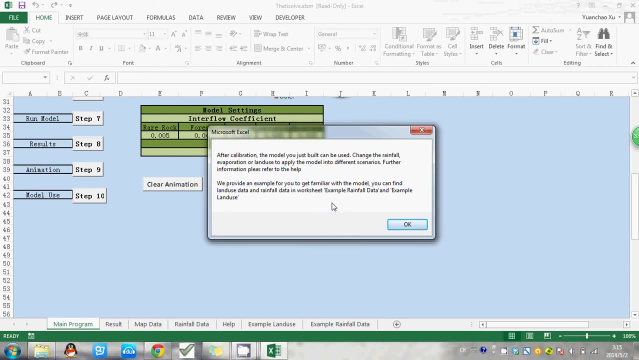 Ok, here we stop the animation, And if you are happy with the animation, just leave it there, And if you are not happy, just clear animation and we will go. Model use Step 10,. we have detailed instructions about how to change the parameters and how to use. 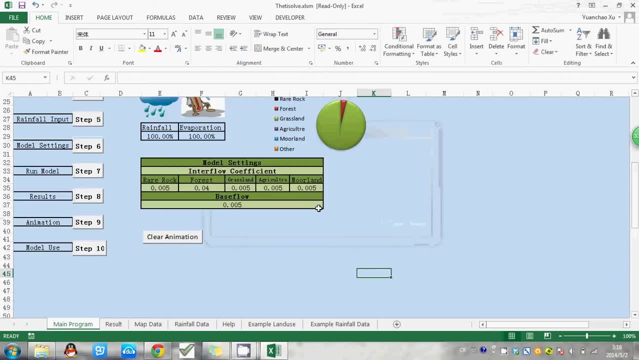 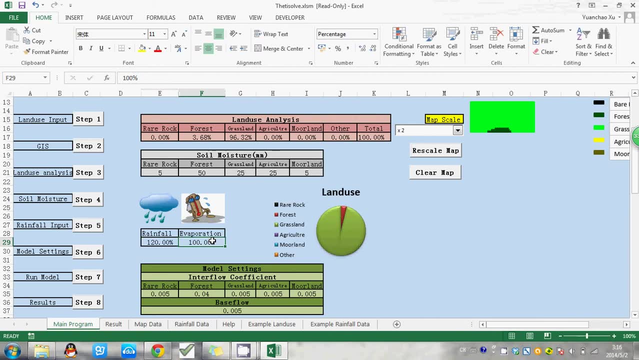 this model to simulate other kind of things. For example, if you want to format the model, you can do that. Ok, Like if you think in future the rainfall will be bigger. like 120% of the evaporation will be less. like only 6% of the evaporation will be taken into consideration. 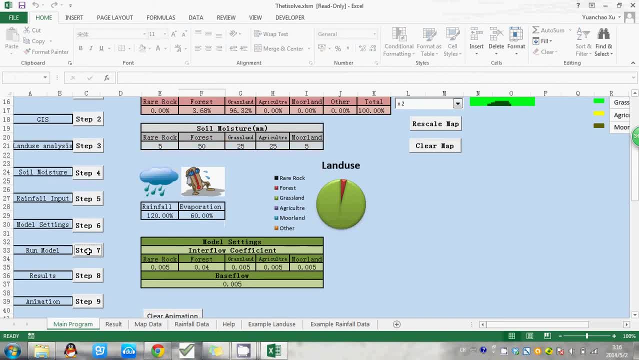 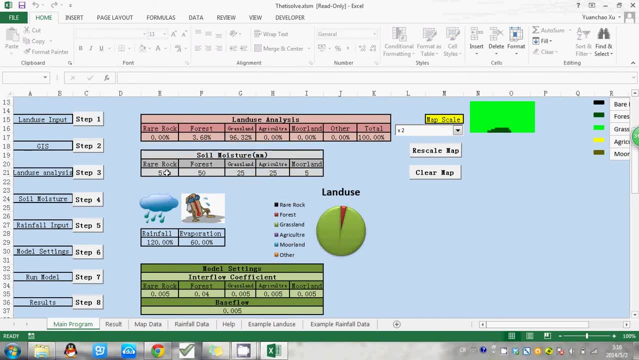 Ok, you can run the model again And it's very fast. And also, you want to see the field capacity is not satisfactory. You can also change here. Also you can change the percentage of the land use, For example. if 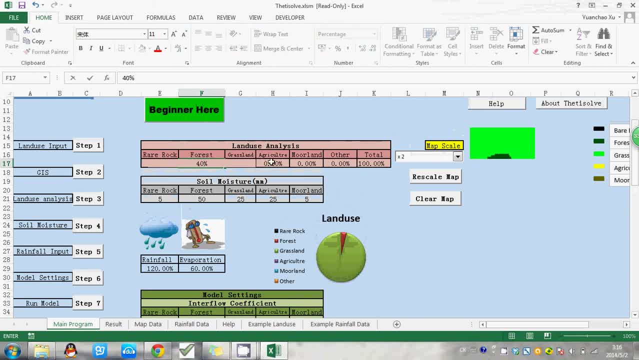 Hi, Hi, Forrester should be more and we can change 40% to here. but remember, when you change here you have to know that the total number should not exist. exit the 100 and so you have to change grassland to 60%. okay, here is now 100. 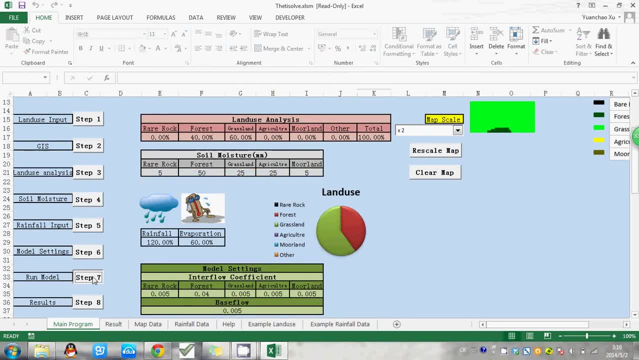 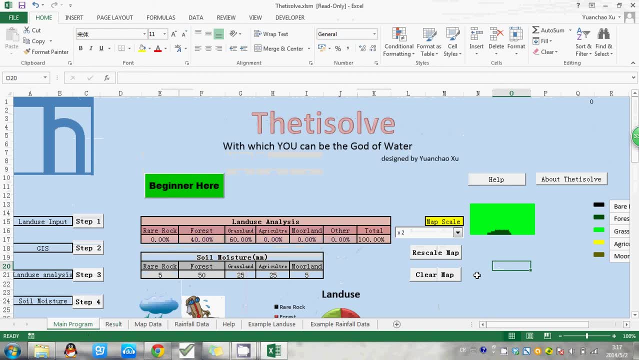 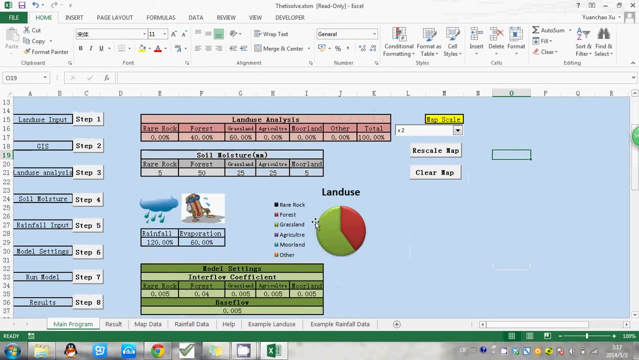 also you can run a model again. you can see the result and you just as the animation. if you're happy with the map, just leave it there. if you're not happy, clear map okay. and if you really want to use this to do some more creative things, 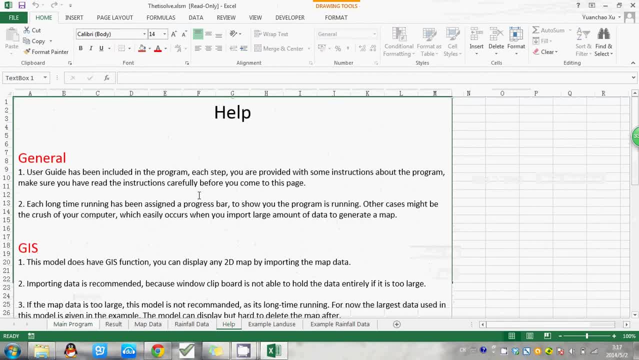 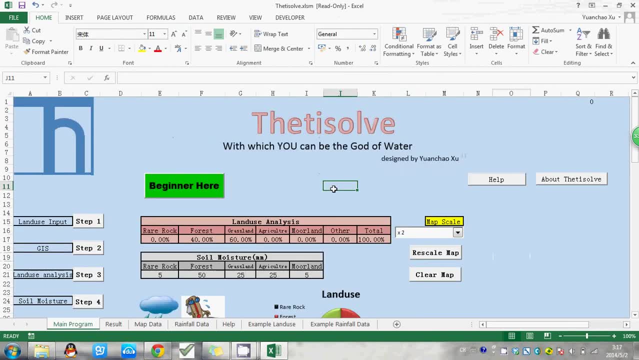 you can click help here. you will get more detailed information about this model and how to change some primary okay. also, if you have some further suggestions or some problems with using this model, just contact me. here is my contact information and thank you for wait for seeing this video. watching this video, okay, sorry.